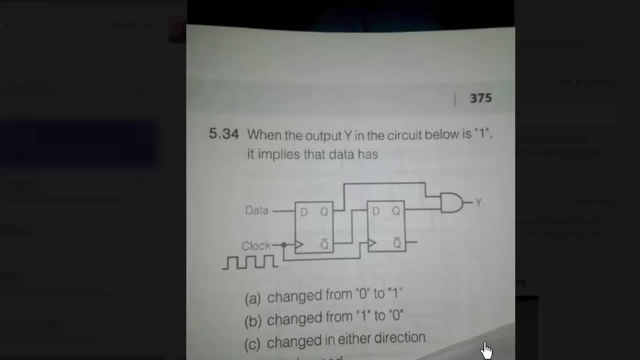 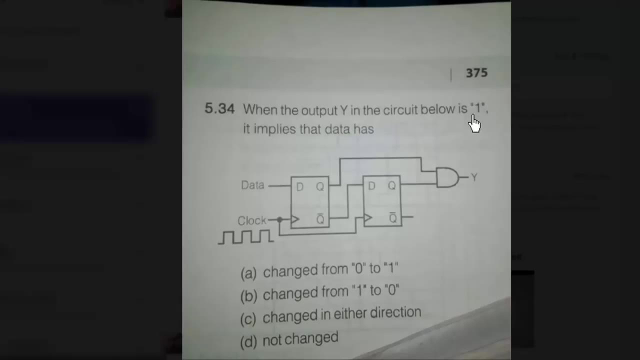 problem, but he needed the explanation. You can see the problem on your screen. Let's read the problem first. When the output y in the circuit below is 1, it implies that data has there are 4 options. according to option A, changed from 0 to 1, according to: 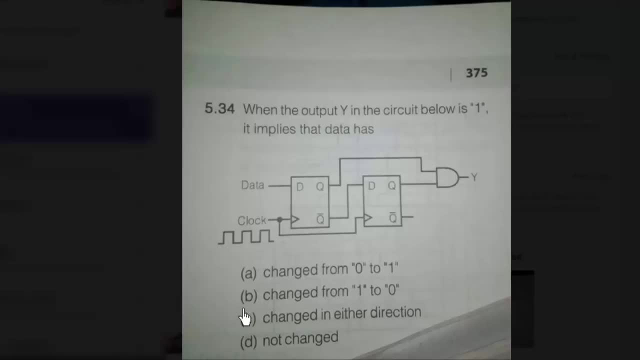 B option, data has changed from 1 to 0,. according to C option, data has changed in either direction: 0 to 1 or 1 to 0. and according to D option- the last option- data has not changed. You can see the circuit on your screen. 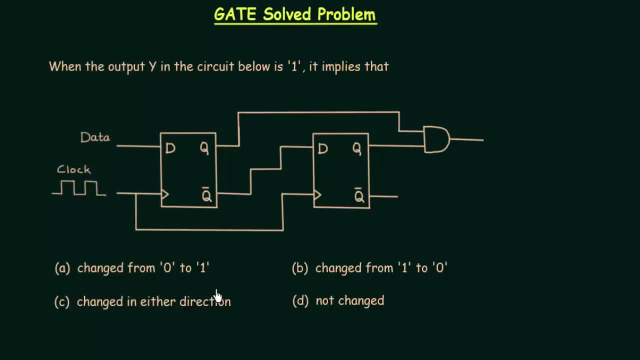 And for better understanding, I have drawn this circuit on my board. This problem is taken from gate 2011 electronics and communication paper. Gate 2011 electronics and communication paper. In this problem there are two D flip flops and one AND gate. The output of this: 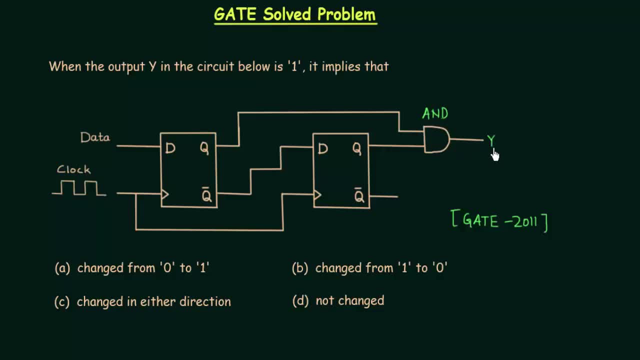 AND gate the output of this, AND gate is y, which is the output of this sequential circuit. Let's say, the first D flip flop is A flip flop, The second D flip flop is B flip flop And because of this reason I will call the input of first D flip flop as DA and the two 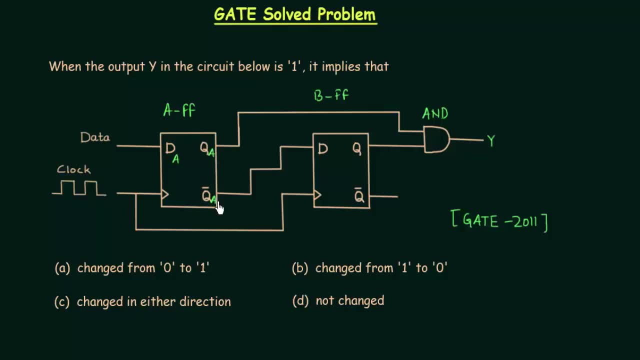 outputs will become QA and QA complement. In the same way, this input will become DB and the two outputs will become QB and QB- QB complement. You can see DB is same as QA complement. The input of second flip-flop, DB, is equal to QA complement and the input of first flip-flop is the data. DA is the. 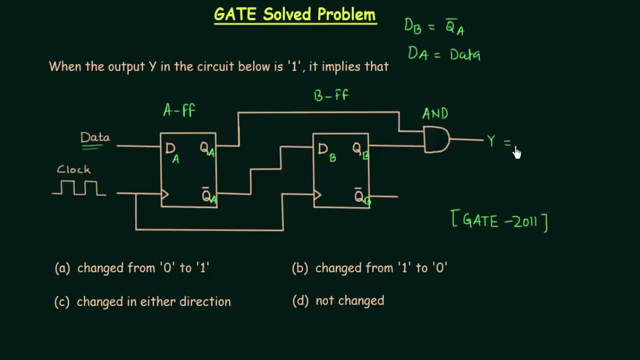 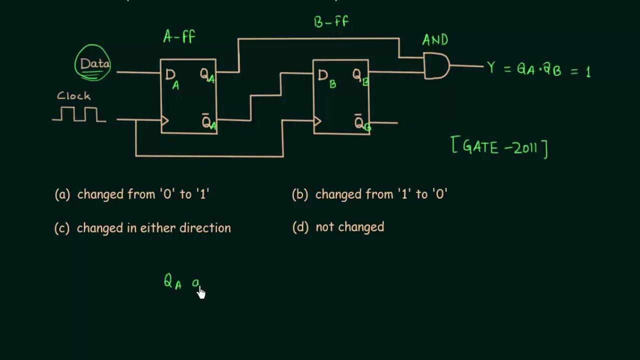 data and the output Y is equal to QA and QB- QA and QB- And in this problem we need to find the change in data when output Y is equal to 1.. When clock is not given to the two flip-flops, then QA and QB will remain in. 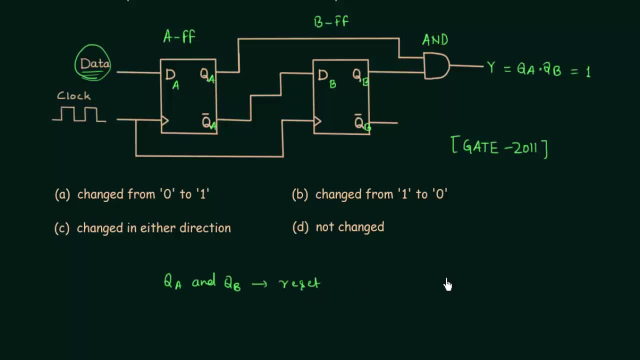 They are reset state. And to find out the correct answer, I will make one table And in this table the first column, the first column is for clock, The second column is for data And the third column is for two outputs: QA and QB. When no clock pulse is given, the two. 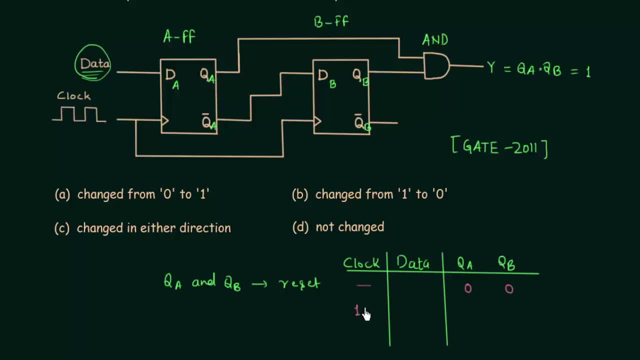 outputs will remain zero. And for the first clock pulse, let's say, data is equal to D1.. Now we will find out QA and QB. for the first clock pulse, DA is equal to data, Data is equal to D1.. This means QA is also equal. 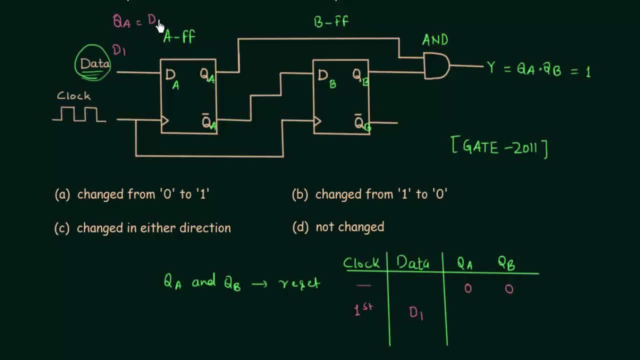 to D1, because QA is equal to DA, Where QA is the output or the next state. So QA is equal to D1.. But this Q1 as QA is only available after completion of the first clock pulse And in case of second flip-flop, DB is equal to QA complement. 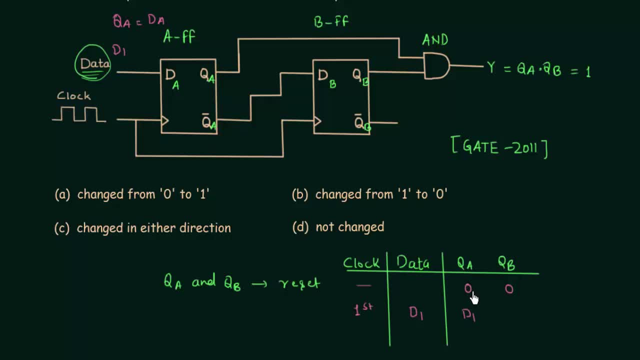 But if you see QA initially, then it was equal to 0.. This means QA complement is equal to 1.. So DB is equal to 1.. This means QB is also equal to 1.. So QB is equal to 1.. QB is not equal to D1 complement, because D1 will be available only after completion of. 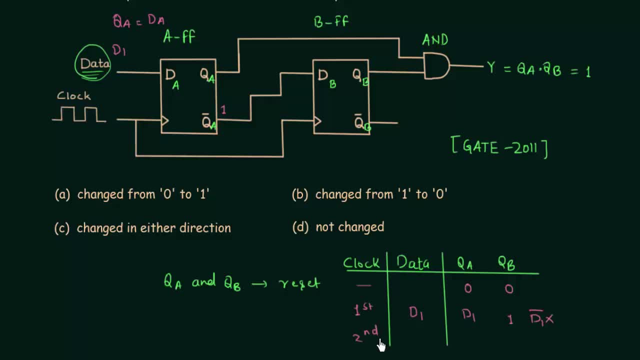 first clock pulse. Now for the second clock pulse. let's say data is equal to D2.. So QA is equal to D2 and QB is now equal to D1 complement. During the second clock pulse, QA is equal to D1.. 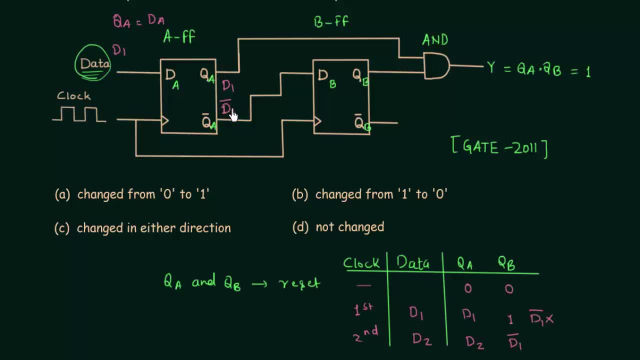 This means QA complement will be equal to D1 complement, So DB is equal to D1 complement and this will make QB equal to D1 complement. So this is the important result from this circuit, And now we will generalize the case. We will generalize the case.